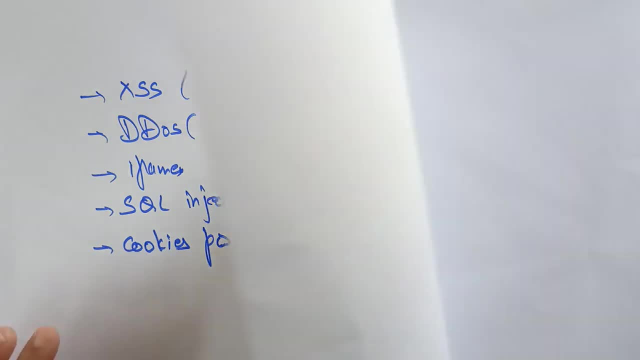 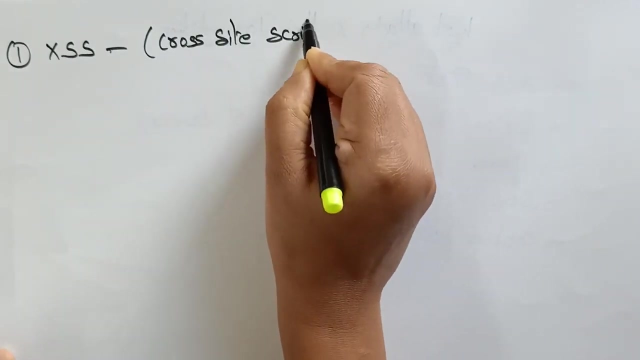 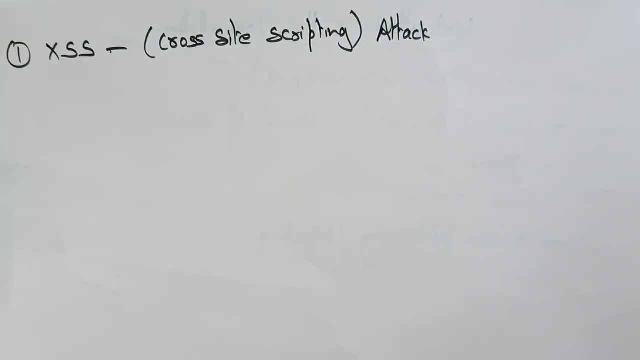 So let's see one by one. So first one is XSS. So let's have a look on this: XSS- Cross site scripting attack. XSS, So what I said. XSS means cross site scripting attack. So like this word, what you are going to understand. So here it is: discuss about the cross site scripting. Okay, So it allows the attacker. Let me write first what is this XSS? It allows attacker, the person who is going to hack the data, So that the person you call it as an attacker, So it allows attacker to inject. 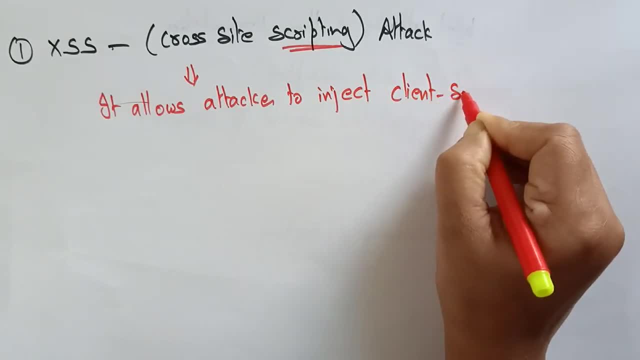 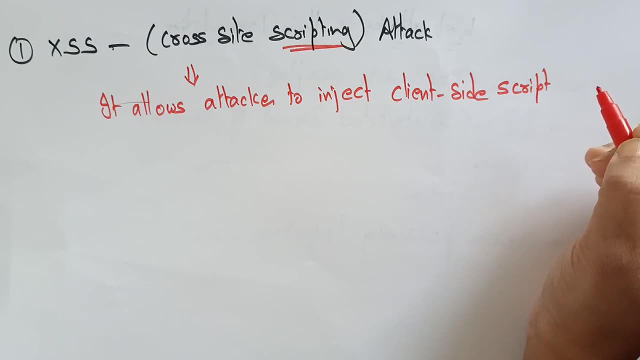 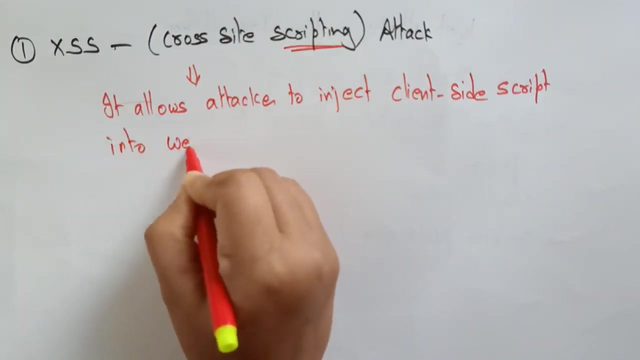 To inject Client side scripting. So you already know about the client side scripting. That is the JavaScript, So HTML. So these are all the client side scripting. So here the XSS allows the attacker to inject Means. he is going to enter some code in the client side scripting That is going to enter into web pages. 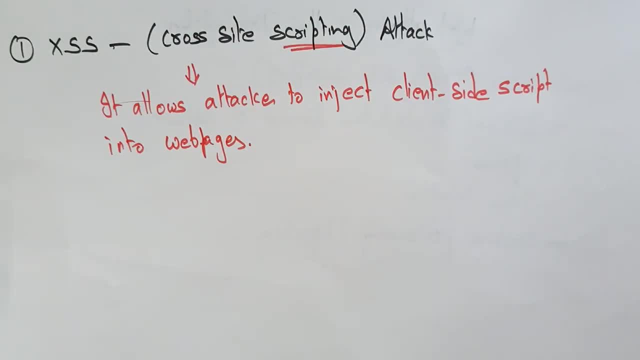 So this is a cross site scripting. Whatever the scripting language that you are writing on the client side, that is a JavaScript. Let's take the example as a JavaScript. In the JavaScript, the attacker is going to inject some malicious code. Okay, So that that malicious code will be entered into the web pages along with the user code and enter into the web server from there to the database. Okay, 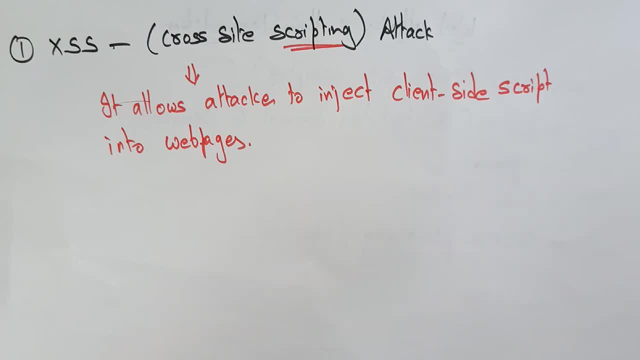 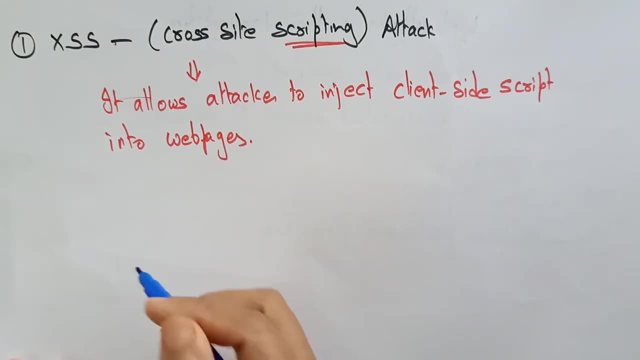 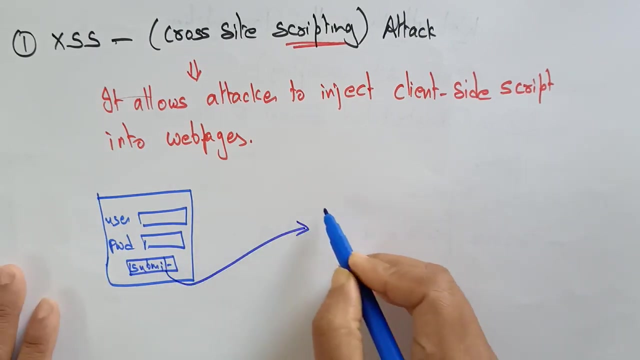 So actually it may be used to bypass the access Control, just for the bypass the access control. Let me explain you with an example. Let me explain you with an example. So let me take the user. So this is a user, The user consisting of the username. So here he is entering his username and he is entering with the password. So whenever these two are entered, he is clicking on the submit button. So what it's generally it is doing whenever they click on the submit button, that page will access the 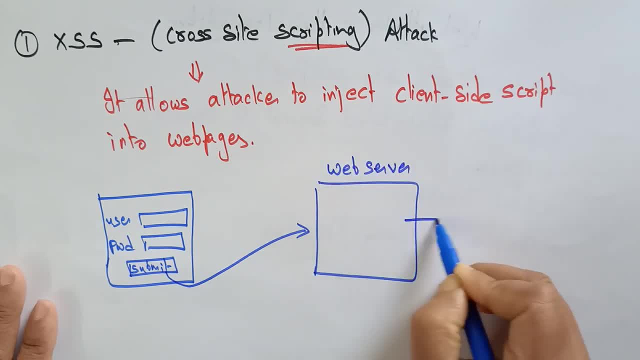 How? So in the web server we are having a database related to that particular person, So it is checking that information, Okay, and the permission is given to that user. So this is what exactly it is having happening. So, in the form the username and password is given, It is validating. the web Search is validating with the data that is present on the website database. So if that username and the password, both all, as say, 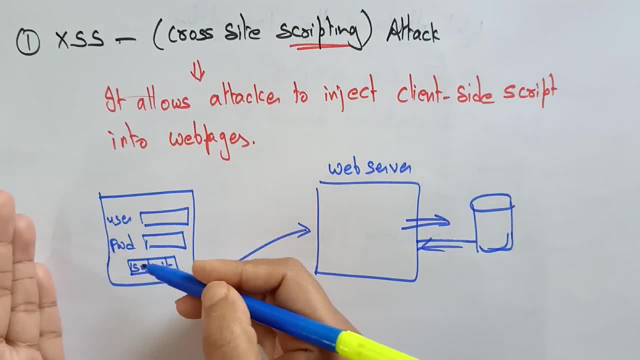 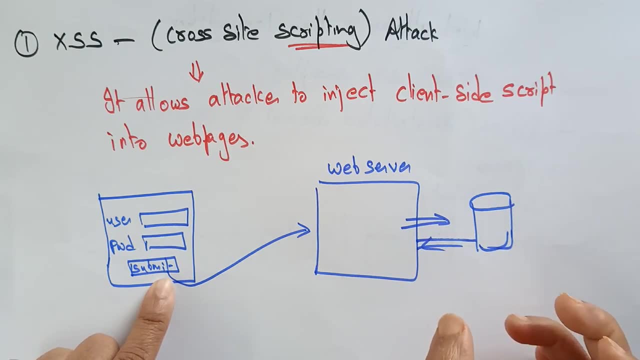 So this is what exactly is happening. Ok, So in the form the username and password is given, It is validating it successful and active. So I Type REPLAY request will be sent. whatever he is accessing that information will again send back to the. 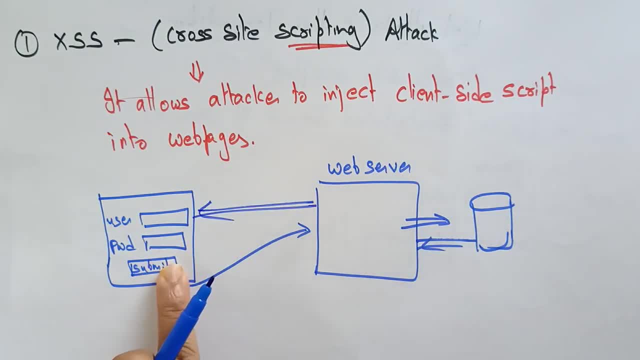 user, the web server is again send that, send back the- whatever the information that user requires, that information will be sent back to the user profile. so this is what happening. so now let's talk about this cross-site scripting, what this cross-site scripting will do. so now the attacker. 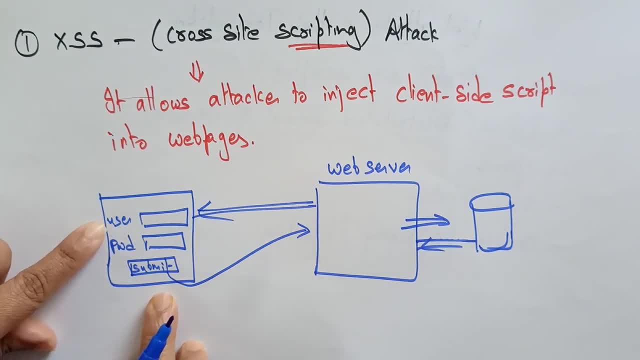 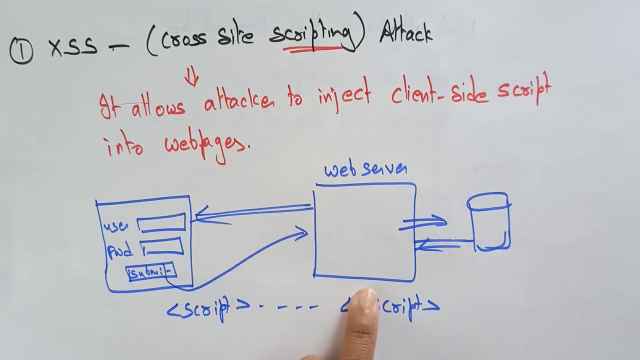 okay. so here, whatever the scripting code that you are writing, like the username, password, whatever the username that you are entering, so along with that, some script code is also, some script code is also entered which contains the malicious code. okay means here in the client-side scripting language, whenever the user click on this submit button. okay, it enter into the web server. that is. 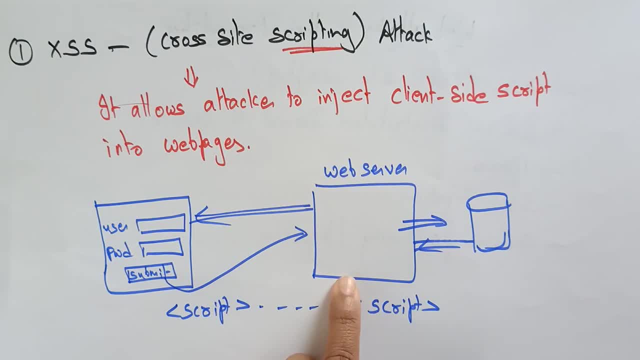 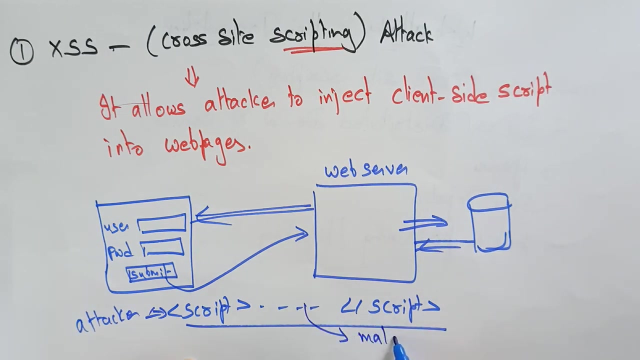 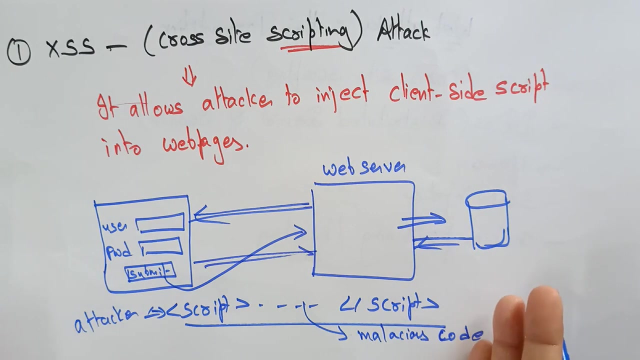 actually the concept. so here the web server simply runs that along with this thing a script is introduced. the attacker, the attacker, add this script, which contains the malicious code- malicious code, so that is also included with this statement, and the web server simply runs. the web server simply runs that malicious code also. then our database or the server gets: 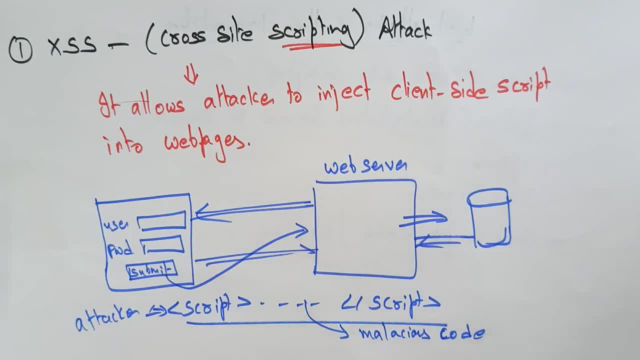 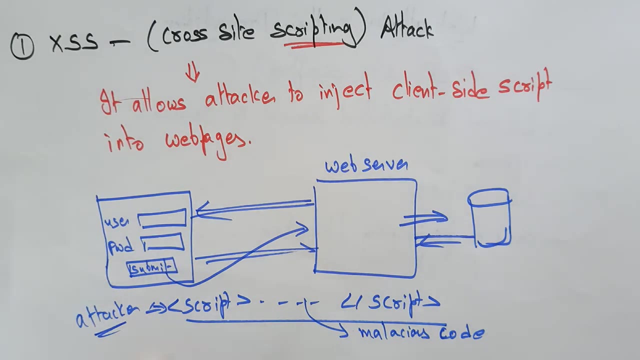 hacked or even it may be damaged also. so this type of web attacks is called as code cross-site scripting. here the attacker is cross-siting whatever the details that is, user is sending. so this is a source that the user can see. okay means anyone can see. okay, open source. so the 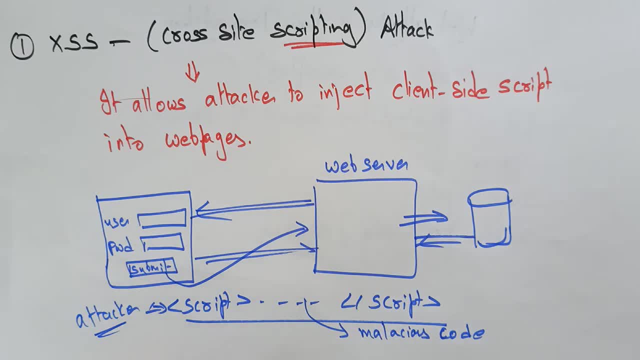 client-side scripting is an open source right. so here the attacker is just entering some information, some script statements in this along with this code. so what the web server will do? a web server will automatically, whatever the user is sending, that it will be accessed. whatever it may be, it will access if it is validated. 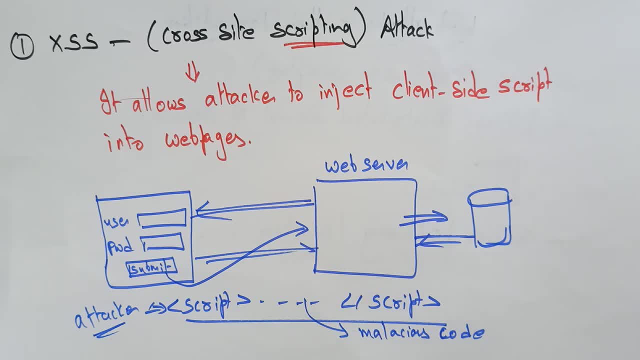 is correct, the it, the validation is right, then, only to produce the required information. okay, it sends the required information to the user. whatever the user is required, okay, so it doesn't know what the malicious code is and what is the correct code and what is the malicious- malicious code that the web server will know does not know about it. so, simply it. 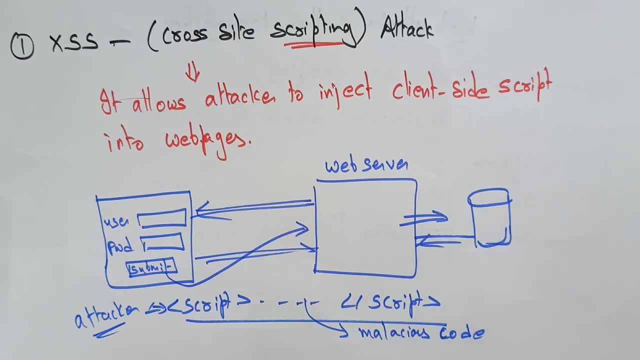 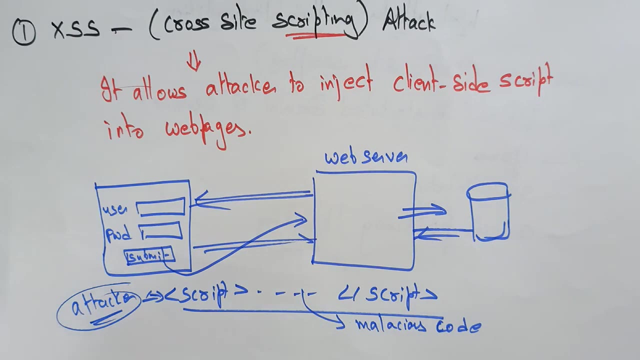 is sending that data to the database and it is getting the data from database. so here the attacker will stealing the data in the database. okay, by cross-site scripting attack. so this is one type of the attack, so where the user, uh, the attacker, can cross-site the 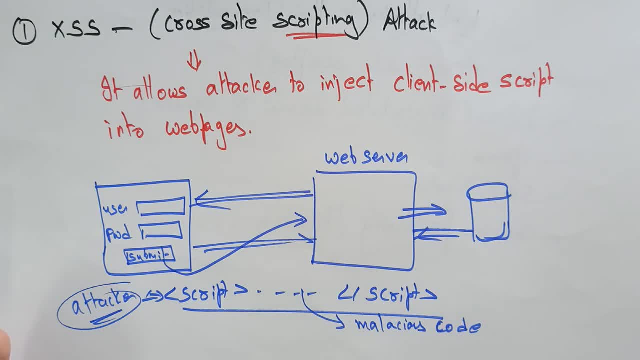 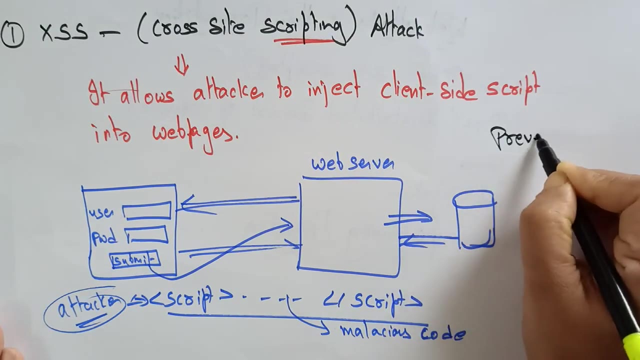 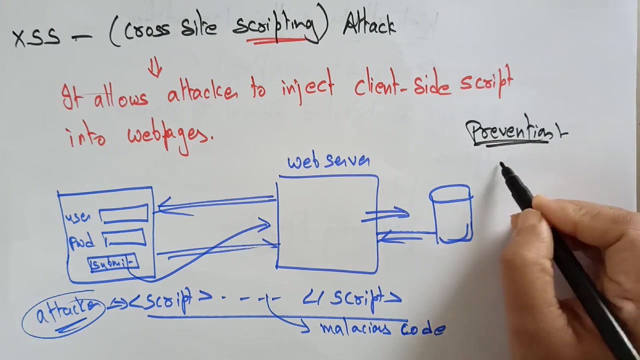 scripting and enter into the database and manipulating the data in the database. okay, so this is a cross-site scripting, one of the web- uh, web server attacks. so what is the prevention for this? how you are going to prevent this? so the prevention for the- how to prevent this cross-site scripting attack- the prevention is: you just need to install. 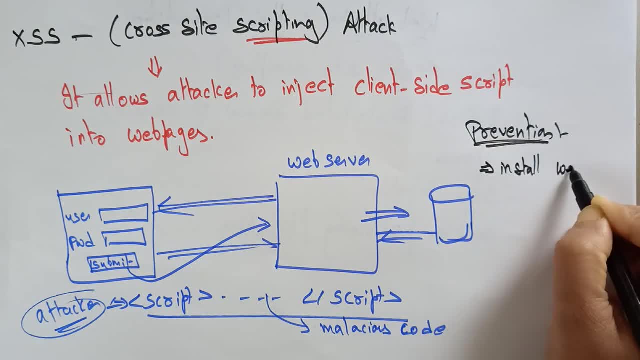 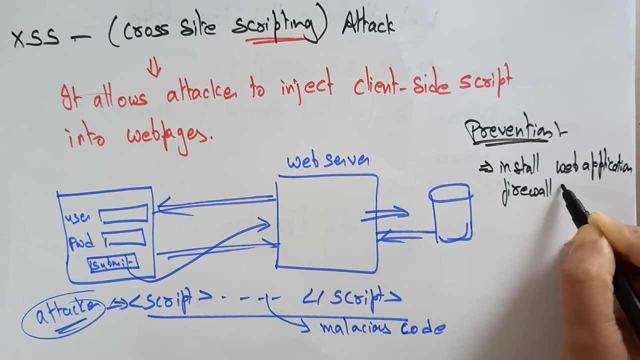 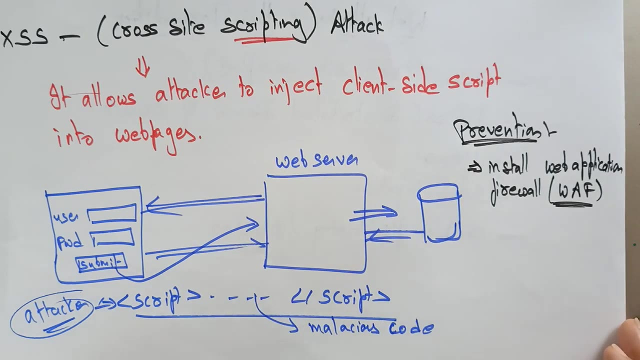 install web application web application firewall. so we need to install the web application firewall, wf, a, af- sorry, the waf- you have to be installed in the web application firewall. so we need to install the web application firewall in your system. install the web application firewall so that it can uh always monitors. 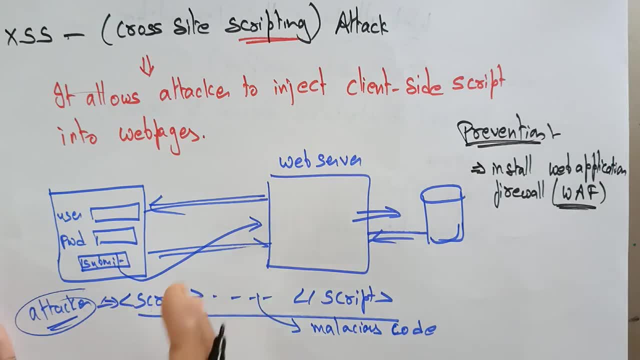 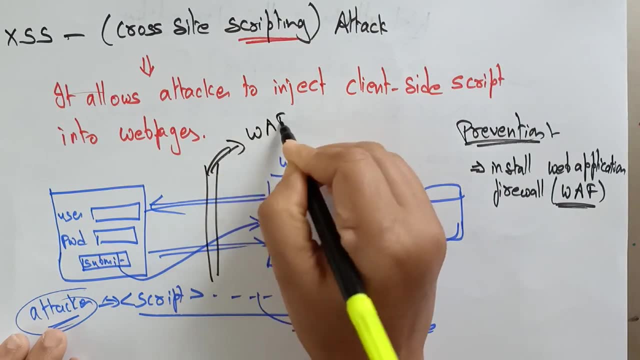 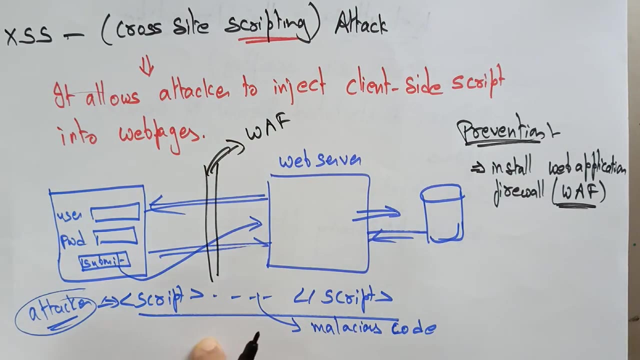 what type of the data that the user is sending, and so that request will be sent to the web server. so in between this, a firewall will be created: waf firewall. so which is the the inst? it is the web application firewall. okay, so now this firewall is going to check what the normal 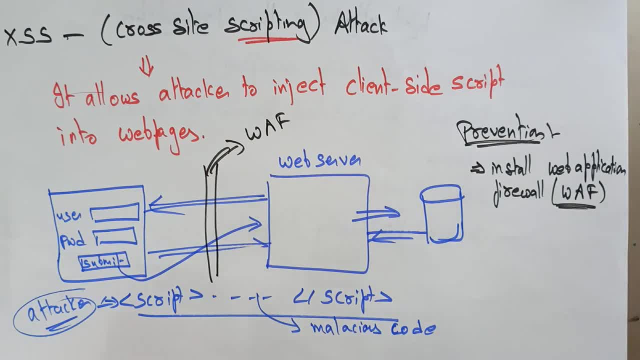 data and what is the malicious code? so it is going to filtered. okay, it is going to filter the filter, the malicious, malicious code or uh, and the normal code. so the normal code will be sent to the web server. okay, so here how you are going to get. is you have to?